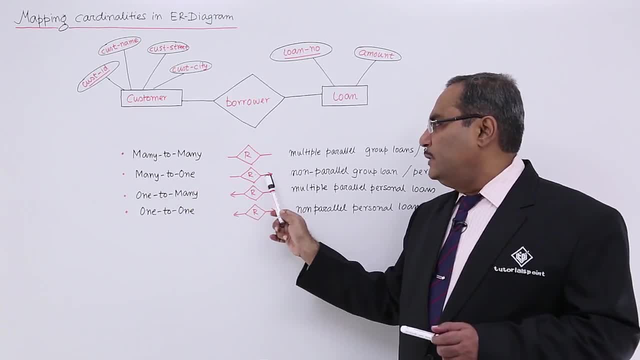 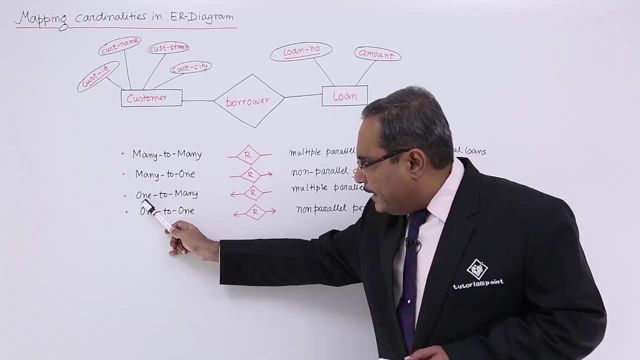 In case of many to one, there will be arrow from this side to that side. Always remember, whenever I am finding one, that side will be one arrow. Whenever I shall be finding one, this side will be having arrow. Whenever we are having one on both sides, then arrow. 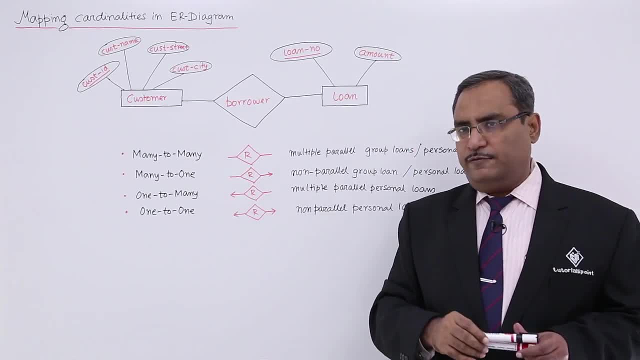 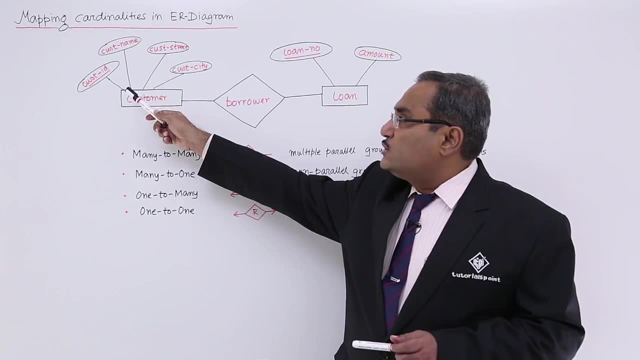 will be there on both sides. Just remember this one. That will be easier For you to understand. So let us go for the first one, That is, the many, to many, Many to many means against one customer ID. we are having multiple loan IDs. That means this: 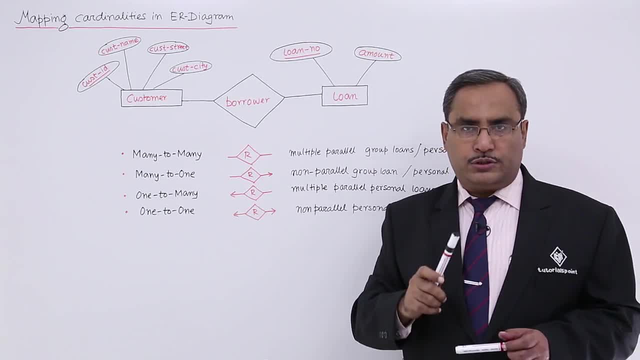 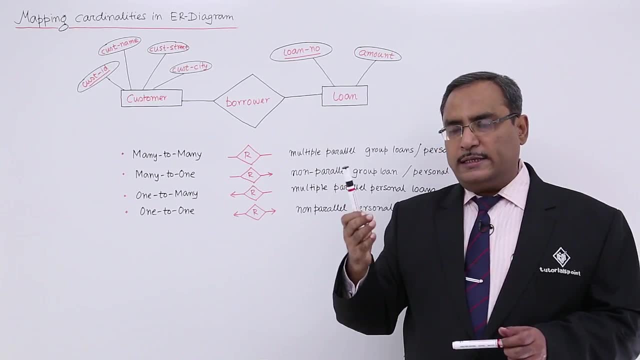 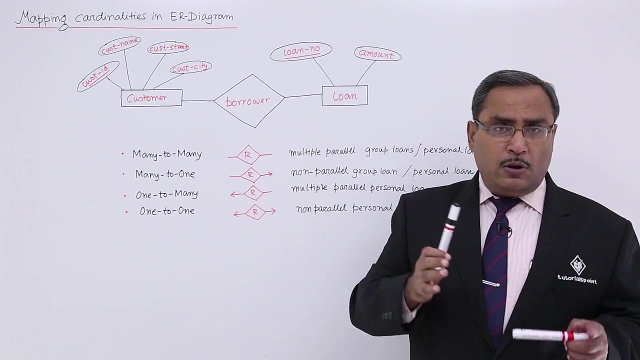 particular bank issues multiple parallel loans. Parallel loan means a customer can enjoy multiple loans. Say one, say one house loan, He has taken one educational loan. I say another one is say some property loan. So in this way mortgage loan, In this way multiple. 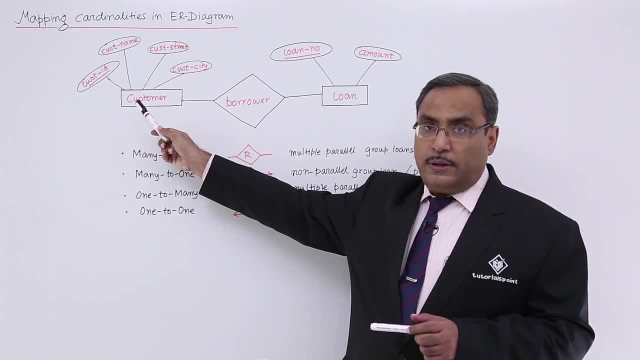 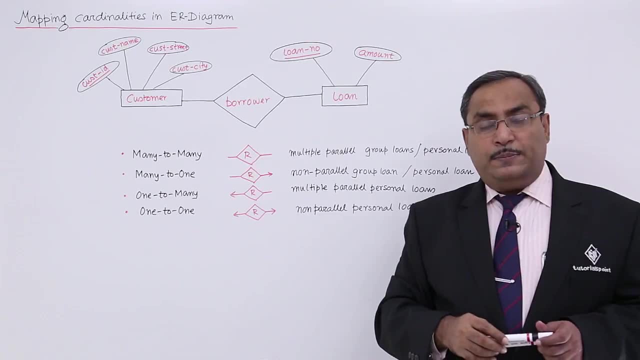 loans this particular bank is Issuing against one customer, But this side is also many. That means against one loan number. we are having multiple customer IDs. That means in case of business loan. let us suppose you and myself has. we have decided that we shall take one loan from the bank. 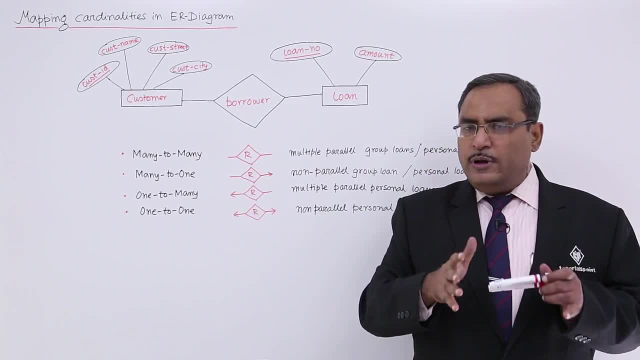 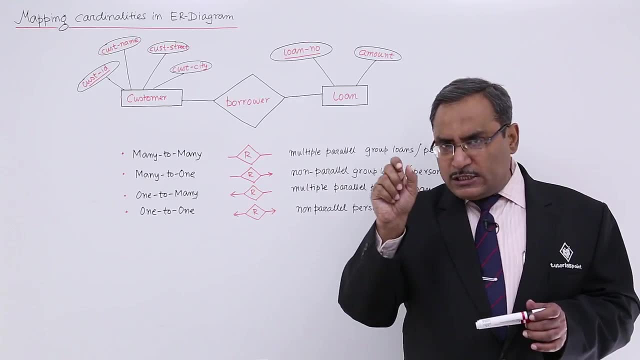 and we shall do one business. So in that case that will be known as a group loan. I am take. I am just considering considering that one as a group loan. So group loan means against one loan number. we are going to have multiple customer IDs. 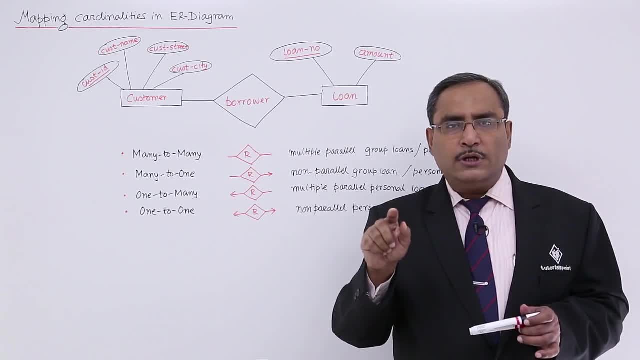 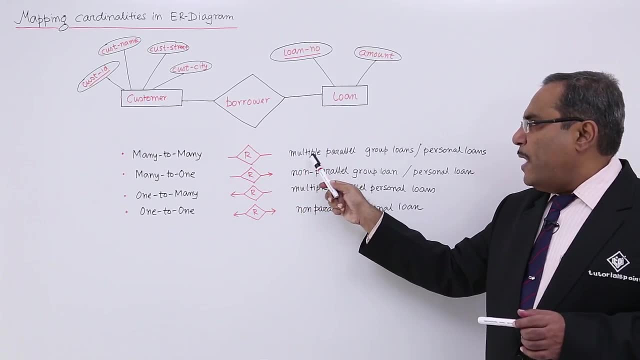 And against one customer ID we will be having multiple loan numbers So we can issue, we can write in this way, this particular bank, in this particular case, many to many- issues parallel, multiple, parallel group loans or personal loans. So in this way we are depicting 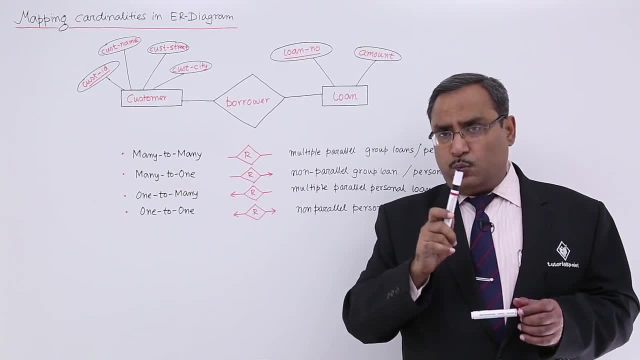 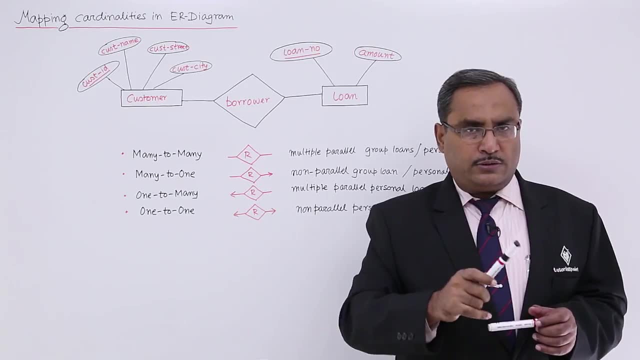 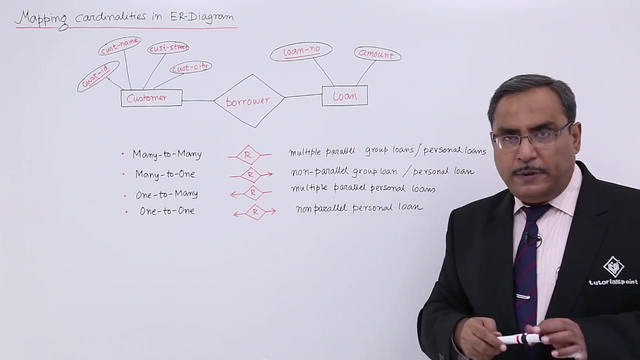 this many to many. That means: against one customer ID, one or more than one loan IDs, Against one loan ID, one or more than one personal IDs. So that is the. that is the respective inference In case of many to one. So let me write that one So many to. 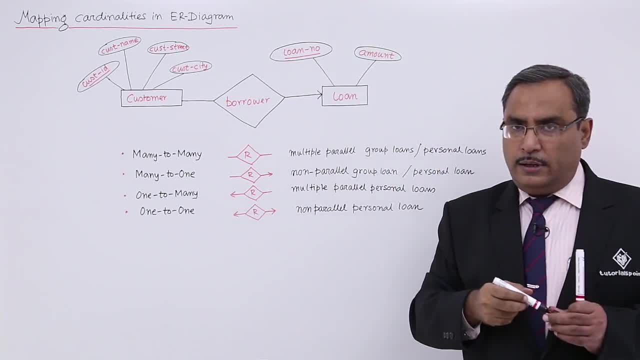 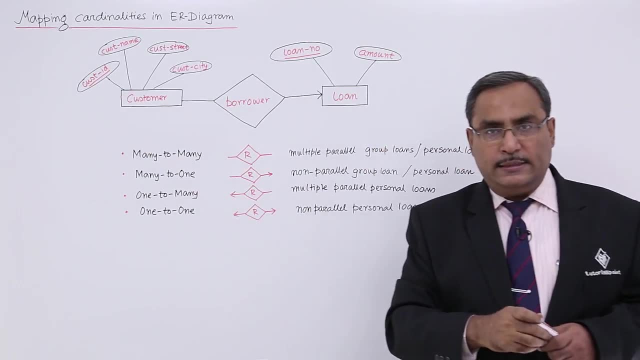 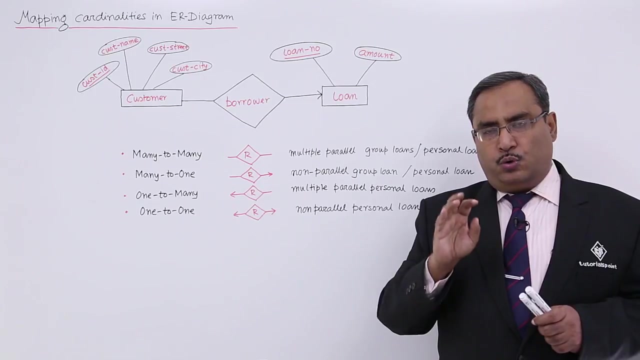 one means arrow will be coming to this particular site. Many to one. That means against loan number. against one loan number we can have one or more than one customer IDs, But against one customer ID there will be only one loan number. That means this bank issues group. 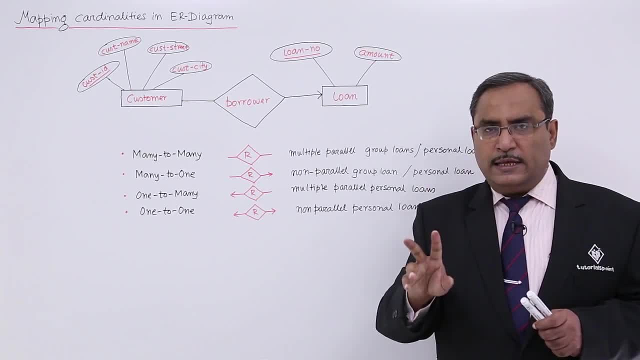 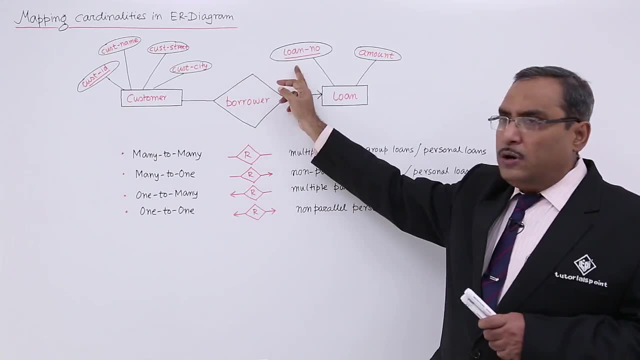 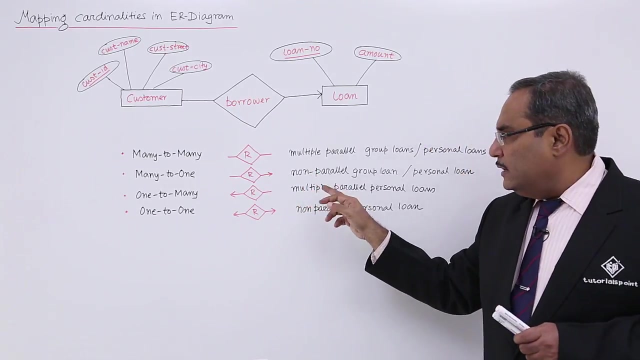 or personal loan, which is non-parallel. That means a customer cannot cannot enjoy more than one loans, Because against one customer ID there will be one loan number, But against one loan number there will be multiple customer IDs. So as an inference I can tell that 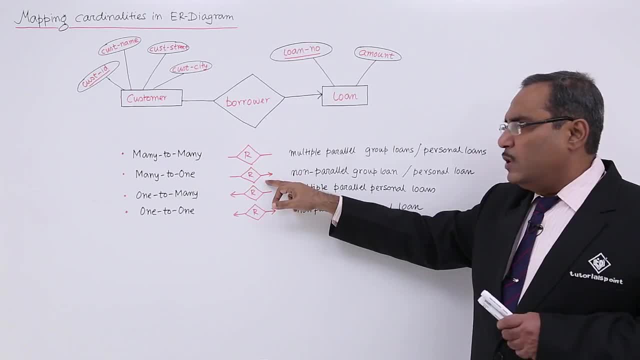 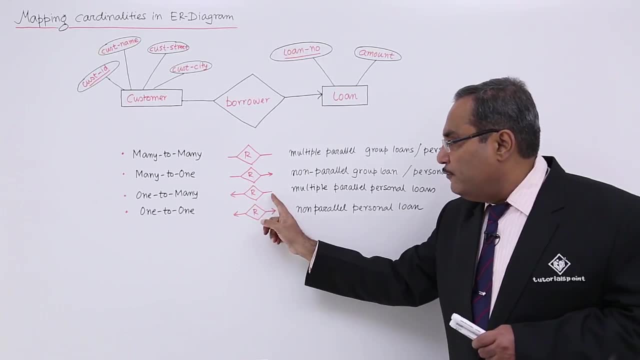 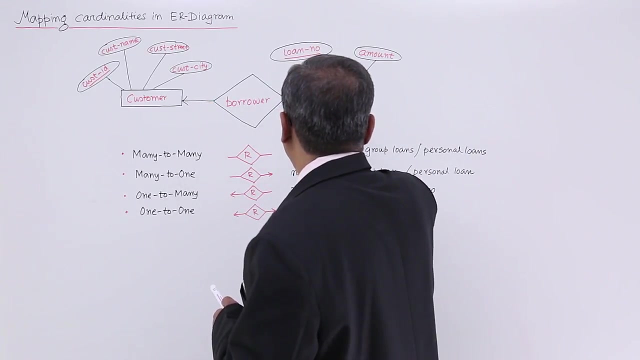 this bank issues. in this particular case, that is, many to one cardinality ratio, non-parallel group loan or personal loan. Next one: we are going for this. That means the arrow will be directed here. That means the arrow will be directed here, So there will be no arrow. 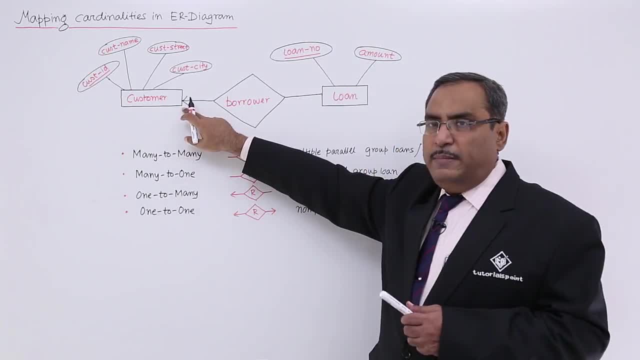 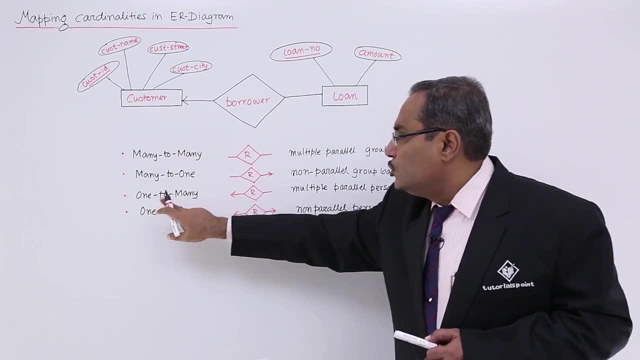 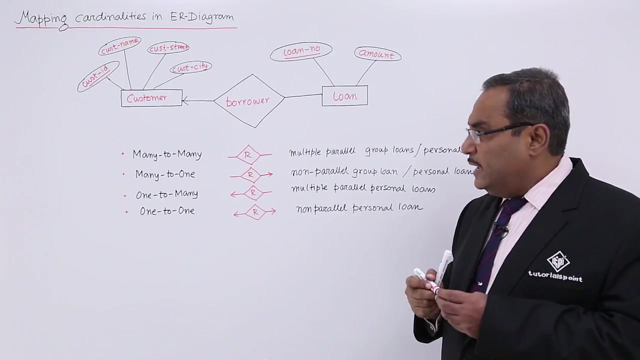 here, Only the arrow will be on this particular site. So this is my many and this is my one. So this is my one. Sorry, this is my one and this is my many, So this is my one and this is my many. Arrow will be directed towards the one. So now, what does it mean? It means: 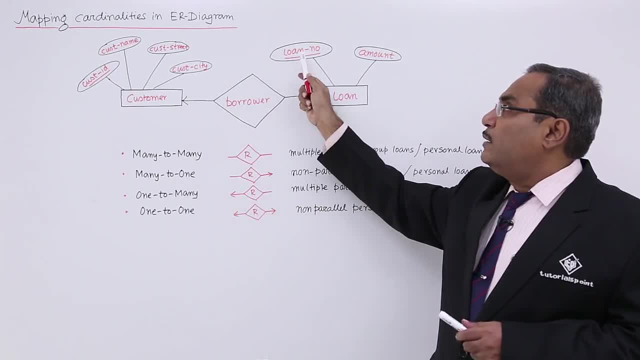 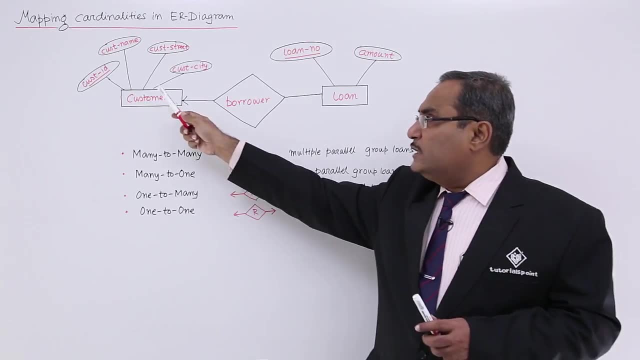 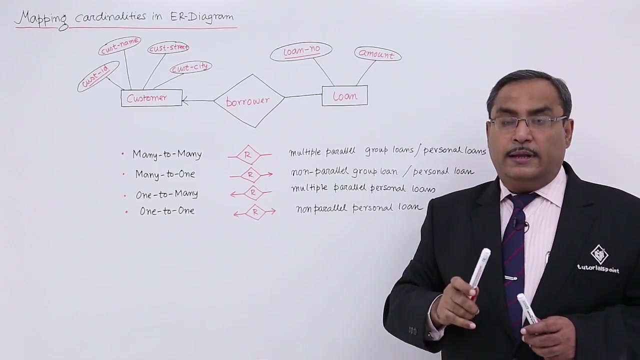 that this particular customer can take multiple loans, but one loan number is having only one customer ID, So one customer ID can have one or more than one customer ID. So that means this bank does not issue any group loan. They issue only the personal loans. So as 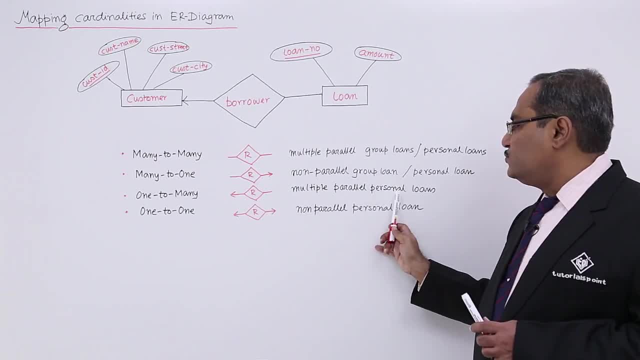 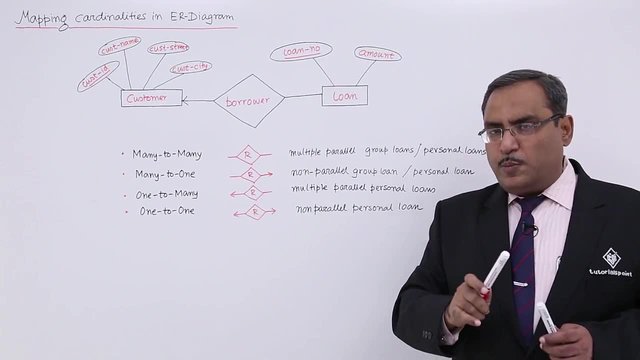 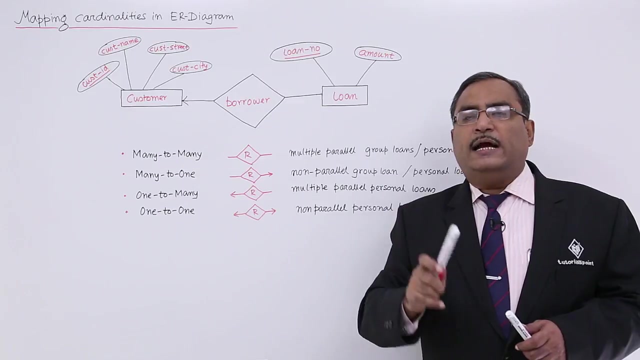 a result of that, I can write multiple parallel personal loans. this bank issues Because against one loan number there will be one customer ID, So it is a personal loan, not a group loan, And against one customer ID we are having multiple loan numbers. That means in. 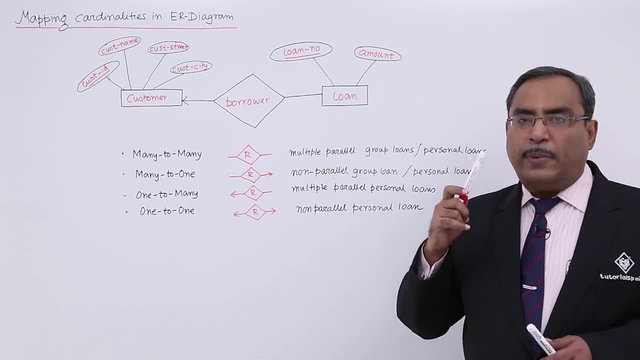 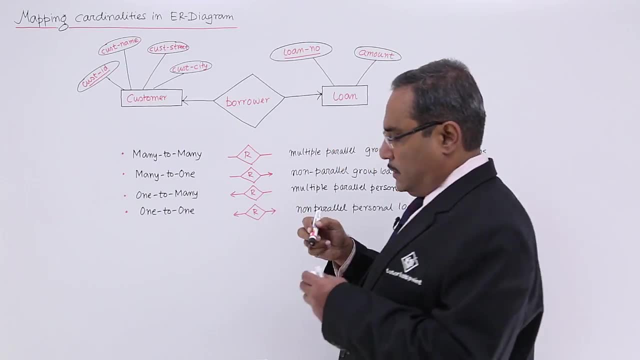 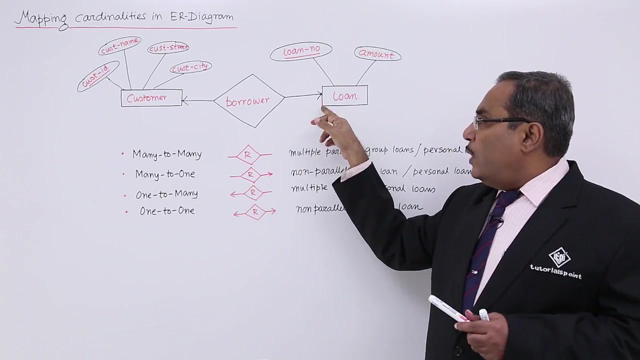 parallel. the customer can enjoy multiple loans, personal loans. Let us go for one to one. In case of one to one, arrow will be on the both sides, So that means against one customer there will be one loan number. So this is a personal loan And against one. 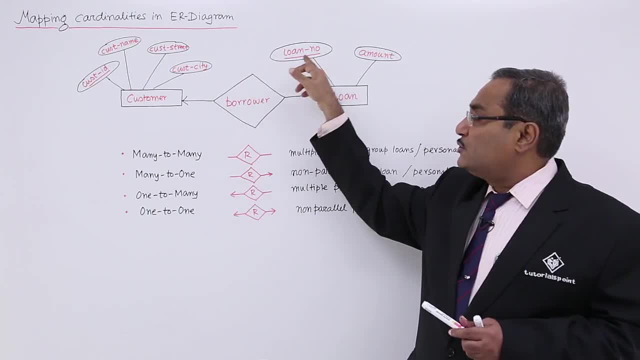 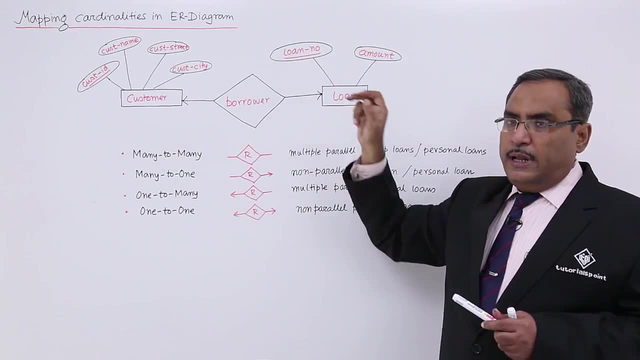 loan number there will be only one customer. So this is a personal loan, Because against one loan number there will be one customer ID And against one customer ID there will be one loan number. That means we are having non-privacy.